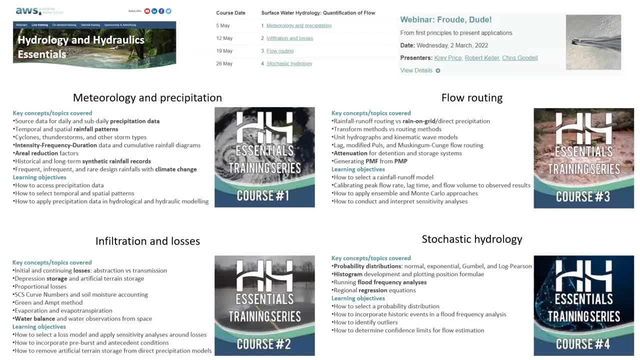 focusing on those things that are most crucial and really trying to make it as useful as possible to you for your work. We'll try to make it as practical and concise as we can And in that regard we've gone and scoured the globe for the most engaging presenters we can find. 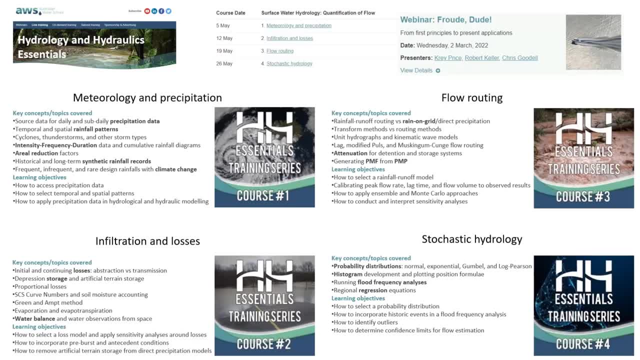 Instructors from across industry and academics. We've assembled a master class for you, using experts From Europe, Africa, Asia, North and South America, And what we find is one of the challenges in teaching water modeling courses that we offer is that we'll get a really wide range of backgrounds in terms of the principles of hydrology and hydraulics. 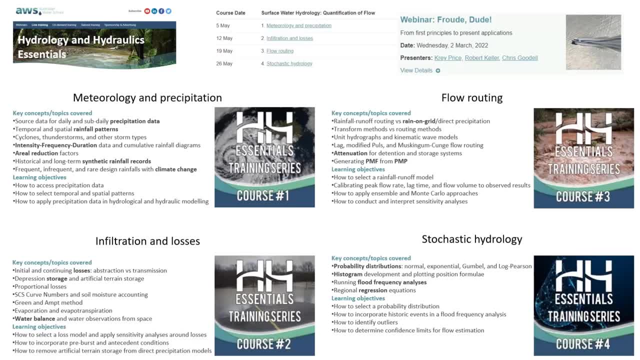 So, whether you're interested in getting just a refresher or maybe filling in some gaps in the background principles that are needed, this course series is geared toward professionals and practitioners in the water space. You will receive continuing education credits for your attendance, But we really think it will be a great experience. 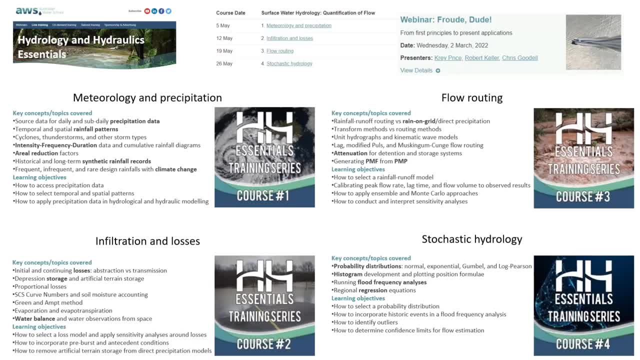 And it will benefit any career in the water sector. So just highlight a couple of the things that we'll be covering. Course one: meteorology and precipitation. What's coming out of the sky dropping onto the ground? taking precipitation data, gauge data and finding out what you need to do to that to plug it into your rainfall runoff model. 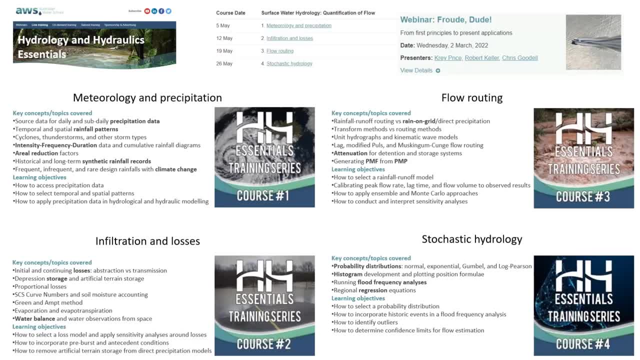 We will cover a full course on infiltration and losses. What happens to that water once it hits the ground? Where is it held up? Where can it get stored? Is it going to be stored in the soil or seeping through the ground? We'll cover flow routers. 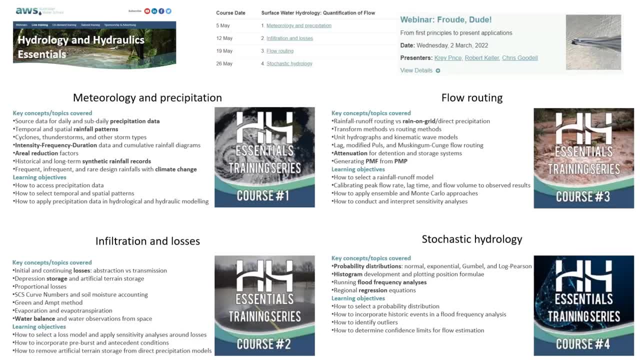 We'll cover routing in course number three, and that's going to involve a discussion about rainfall runoff models in a routing model versus a rain on grid model, which is becoming more and more common these days. We'll talk about the probable maximum flood, probable maximum precipitation and selecting a model and calibrating the peak flow rates. 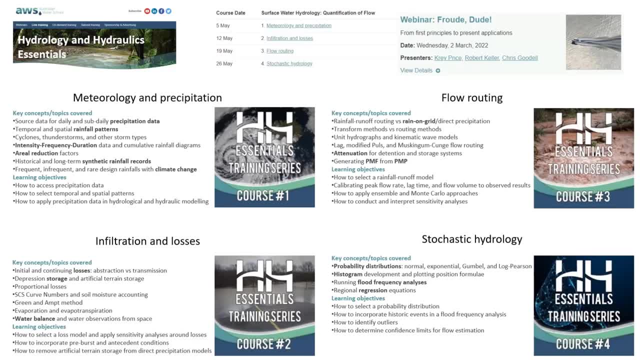 These all involve hands on practical applications with workshop exercises where you can try out the principles that we explain. Our fourth course is on stochastics and turning things into frequency analysis, So we're going to talk a little bit more about that in just a moment. 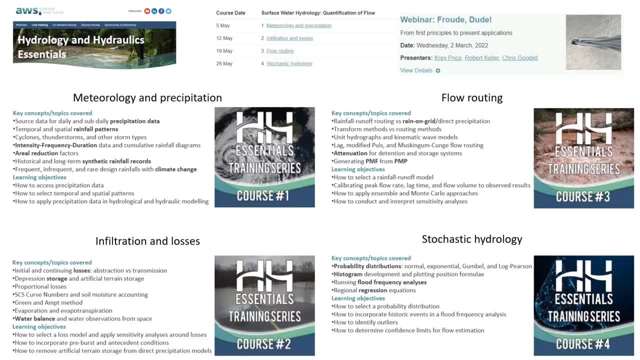 So we're going to talk a little bit more about that in just a moment. And what do we mean by annual exceedance probability or average recurrence intervals and things like that, Taking regression equations and plugging those in with our flood frequency analysis and developing histograms? 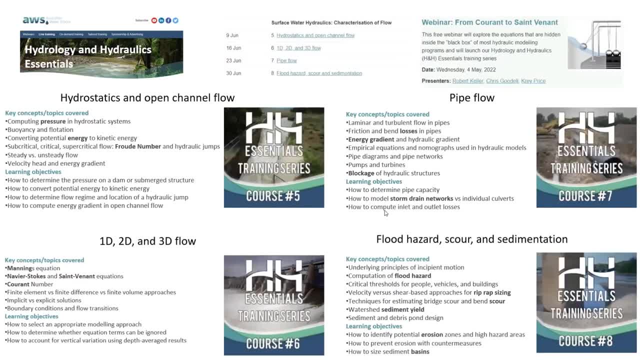 So that rounds out our surface water hydrology courses. We'll then move into surface water hydraulics, starting with hydrostatics, just standing water, What? what are the pressures look like? Then we start moving that standing water and converting the potential energy into kinetic energy. 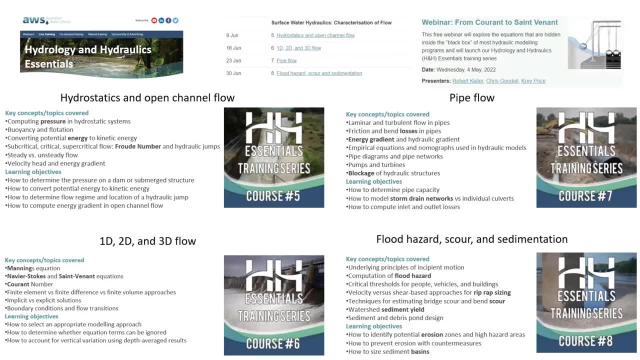 We'll explain the Froude number And key concepts involved in open channel flow. We'll then get into 1D, 2D and 3D flow- Some of these terms that get bounced around, that sometimes are hidden in the black box of the program. 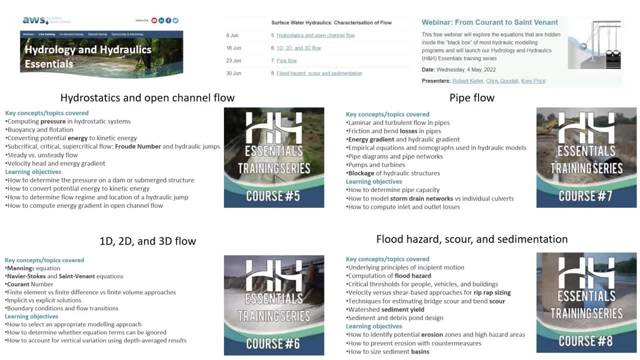 We really want to make these accessible to you and we'll cover some of the key equations: The Manning's equations, Navier-Stokes, St Venat will address the Courant number and other really important concepts to grasp in selecting whether you want to do a 1D, a 2D or a 3D approach. We will also cover pipe flow. That will be covered in the next class. We'll then get into 1D, 2D and 3D flow. We'll then get into 1D, 2D and 3D flow. 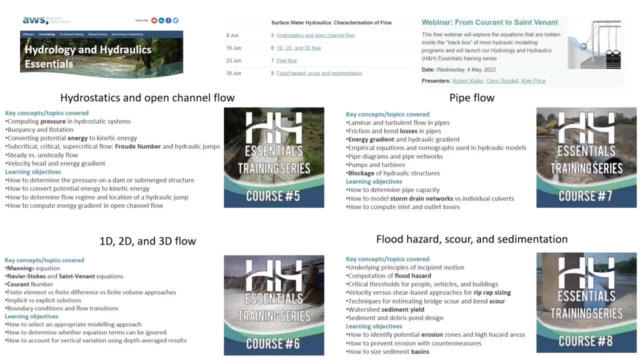 That will include developing energy gradients and hydraulic gradients for pipes. And finally, our last course of the series will cover the flood hazard scour and sedimentation. Get into riprap sizing and some of the scour And we have in a lot of these more detailed courses that are available. 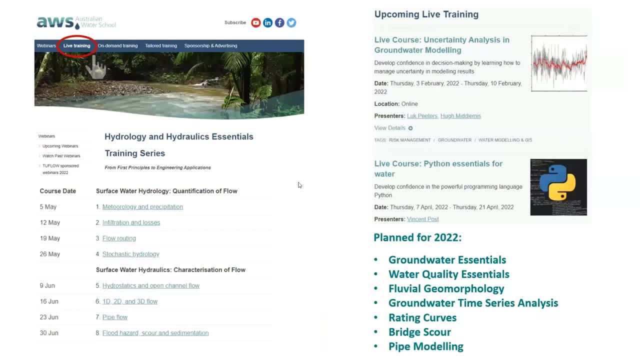 But this really is intended to get you just the details that are needed to get you going. So we're excited again to be offering this and that registration link, as I said, is live now. We'd love to see you online And with that I'll turn it back to Joel. 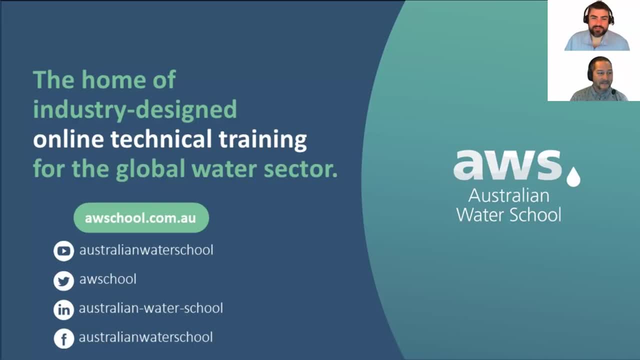 Thanks, Craig. We really appreciate that introduction And hopefully we will look forward to seeing you online. So each of those courses are three hours long, So we encourage you to sign up as soon as you can to the live courses. That way you can get interaction and discuss things live with the presenters that are online. 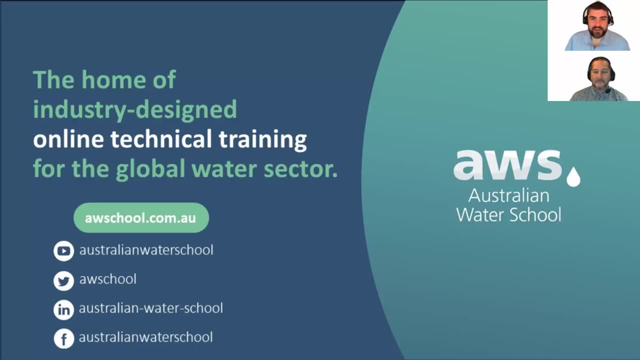 Otherwise, if you cannot attend live, you can always watch it via the recording. Each of the courses will be uploaded to a learning platform where you can download course materials. You can go back and watch the recording As many times as you like. you'll have four months access to each of those courses, up until the end of September for the live courses. 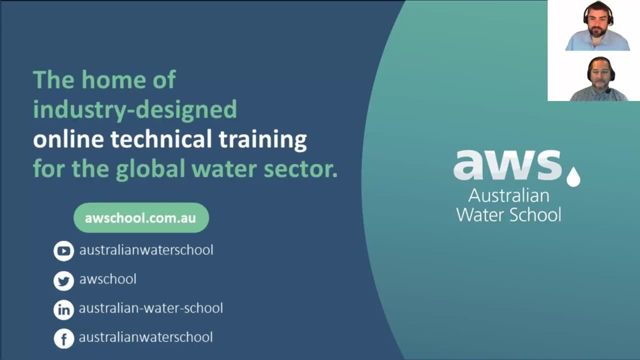 And then, from there on, if you sign up for the full series, you get access for four months. We look forward to seeing you online. It's really exciting and a great initiative to be headed by Craig here as the lead presenter in it. So thanks again and see you online in 2022.. 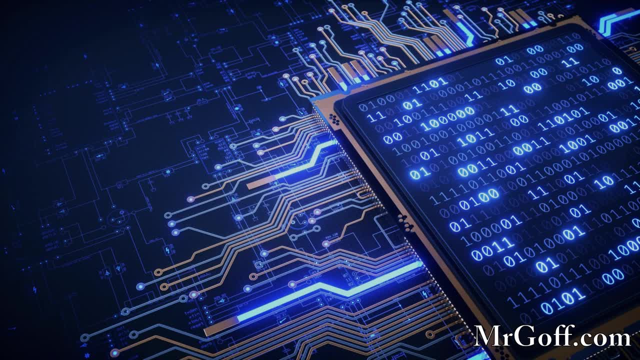 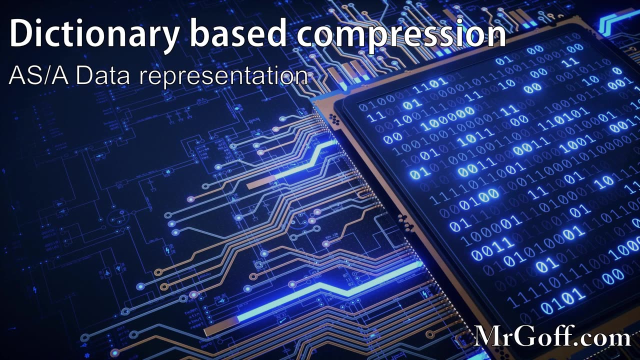 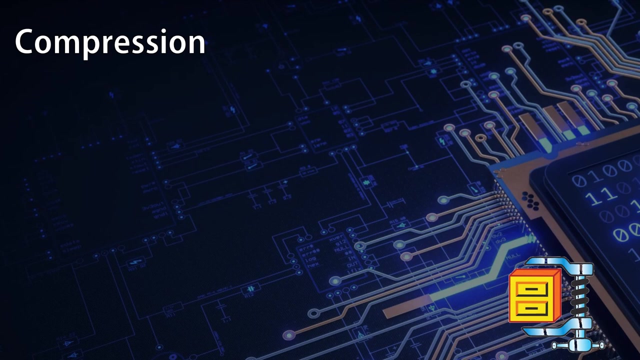 Hello and welcome to another A Level Computer Science video with me, Mr Gough, for MrGoughcom. This video will focus on Dictionary Based Compression. Before we start looking at Dictionary Based Compression, let's do a quick recap of the stuff you should know about compression from GCSE. 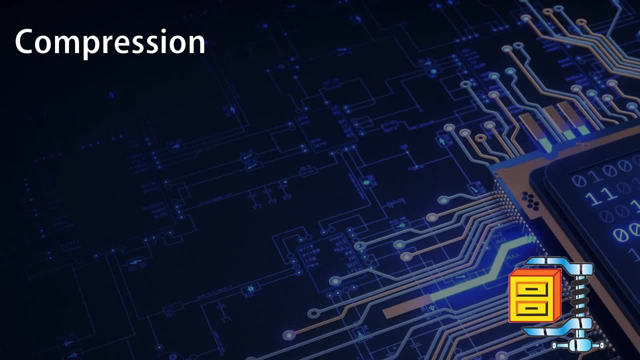 Once again, if you didn't do GCSE, you should go back and look at this compression stuff first before trying to learn about Dictionary Based Compression. So to start off with our recap, compression is the process of making a file smaller in size. 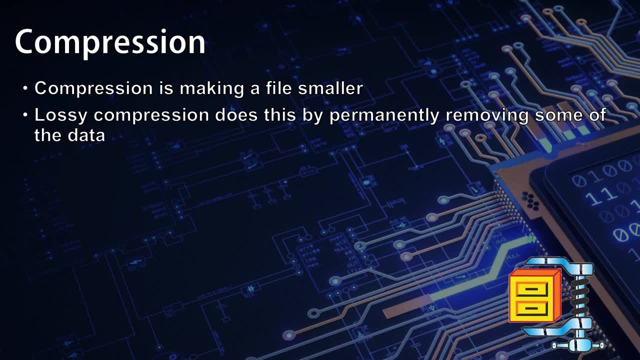 Lossy compression does this by permanently removing some of the data, Obviously with a text file. this would be a problem because when it's uncompressed or decompressed then you can't get the exact same data back again. Lossless compression achieves compression without losing any data. 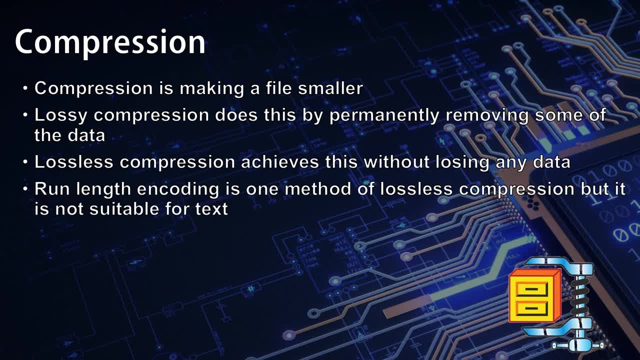 We learned at GCSE about run length encoding, and it's one method of lossless compression, but it's not suitable for text, because it needs runs of the same character to happen one after each other. One possible solution for compressing text that is lossless is to use Dictionary Based. 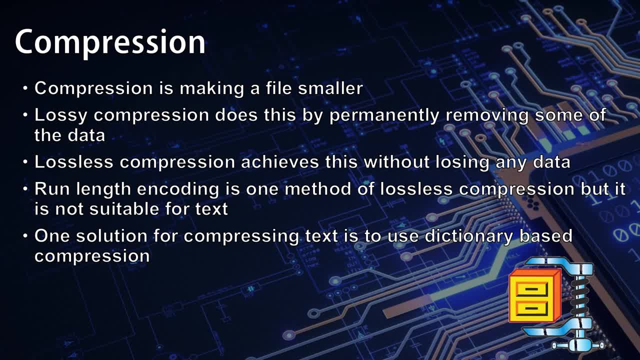 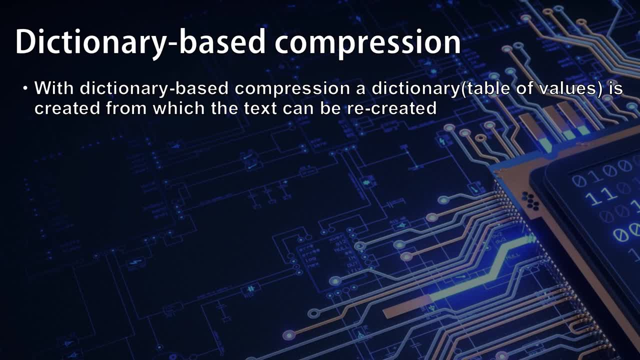 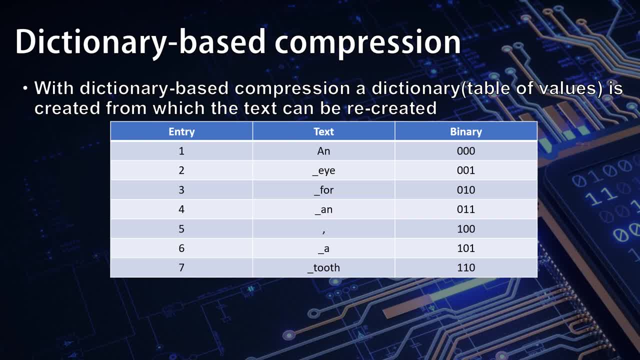